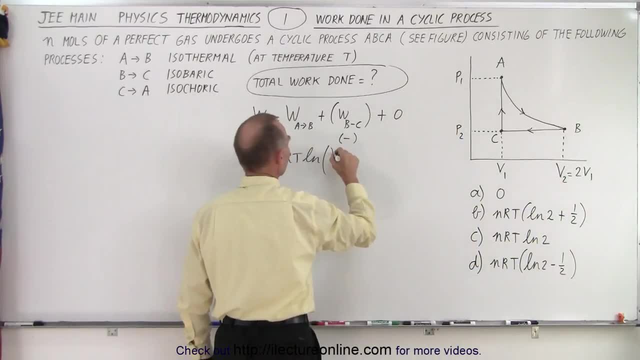 volume, that would be v 2 over v 1, so v 2 over v 1, and since v 2 is twice v 1, this would be equal to nRT times the natural log of 2.. Or we can replace nRT by pressure 1, vol 1,. 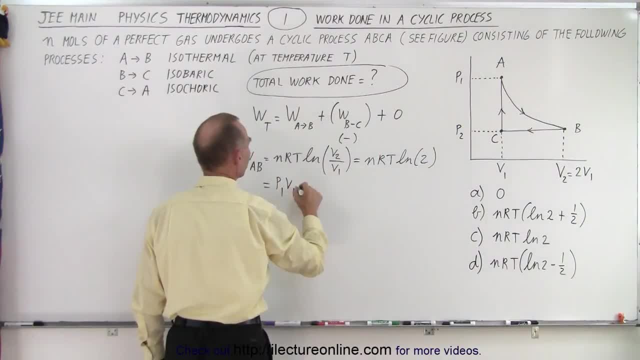 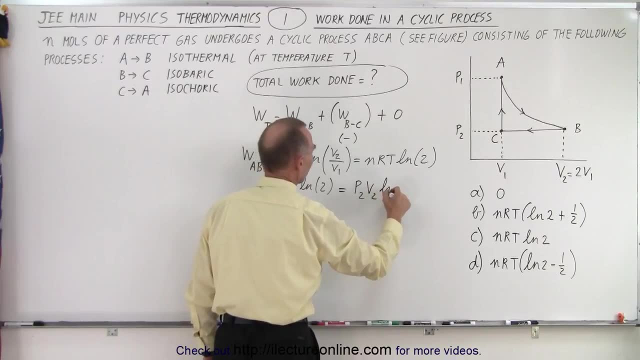 so this can also be written as P1 v1 times the natural log of 2 and that can also be written as P2 v2 as the natural log of 2.. The first one is i times i, i, and this is the projection volume. So if we put it into, 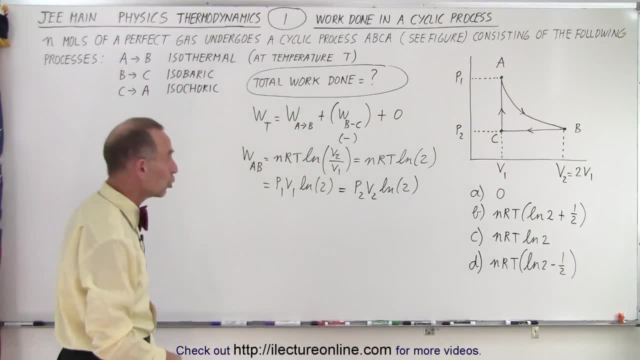 0, it is zero. I've already spoken of the version in 1,, since i times i and nothing log of two. so those are the three possible equations we could use. all right, so next, and let's see here, since the answers are in terms of NRT, then 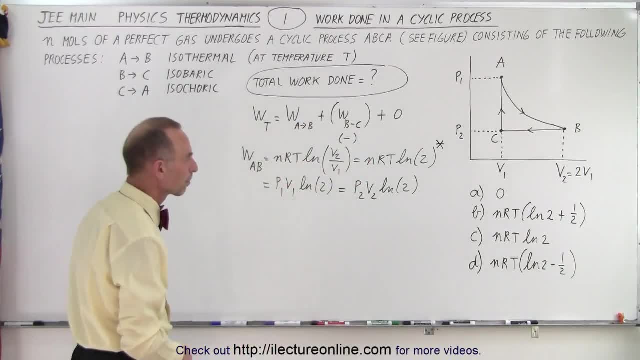 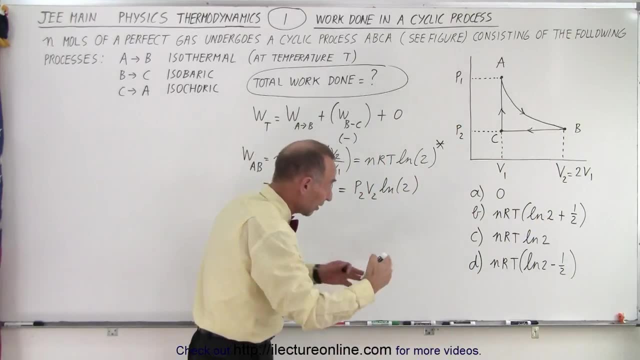 this would probably be the right equation to use. all right, what about the work done going from B to C? now we know that's going to be negative work, because we're compressing the gas, we're doing work on the gas. so the work done from B? 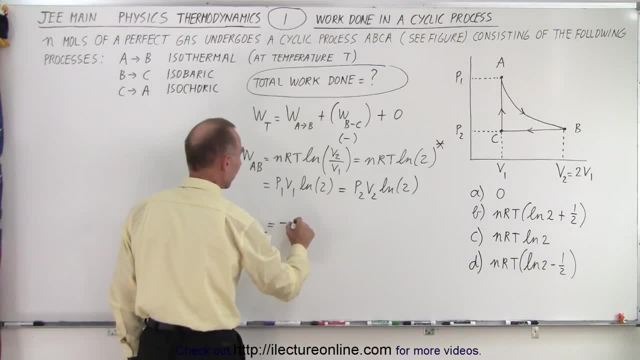 to C is going to be equal to the negative of the pressure, which is constant. in this case it's P, two times the change in the volume, so times the volume change, which would be V 2 minus V 1 or better yet the negative sign can. 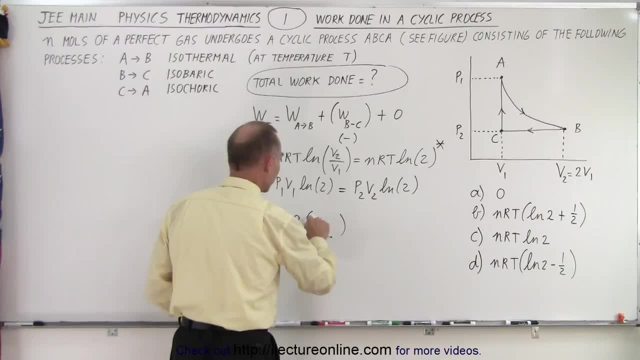 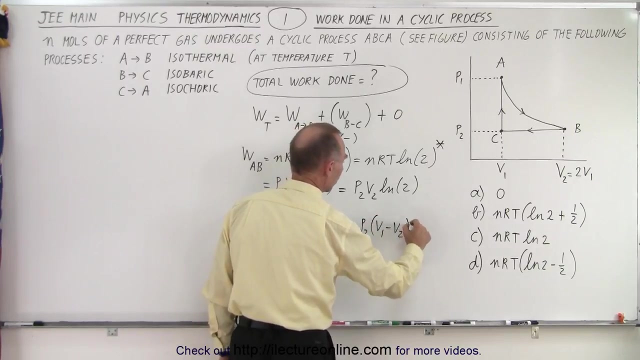 actually be taken care of by simply getting rid of that and simply doing V final minus V initial, and of course V final is V one in each. initial is V 2, so this would be P 2 times V 1 minus V 2, which is 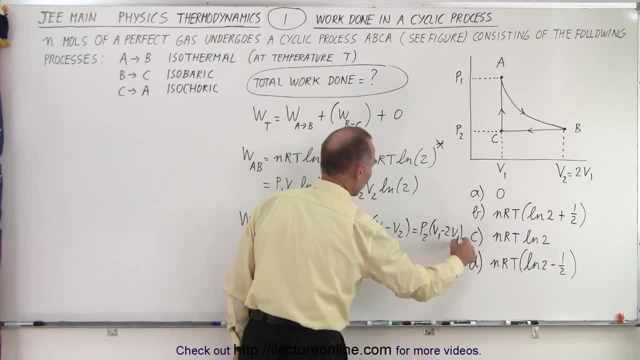 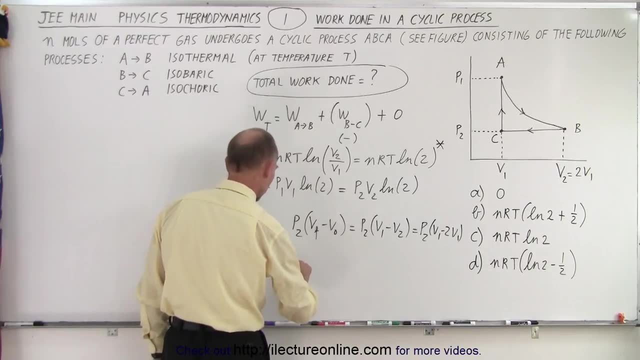 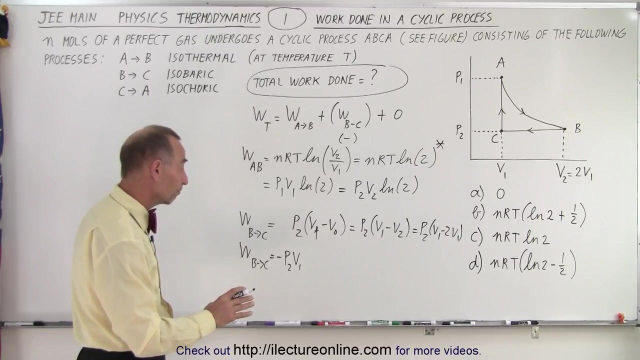 equal to P 2 times V 1 minus 2 V 1. so in essence, the work done going from B to C is equal to P 2 or actually a negative- I forgot the negative there- and negative P 2 times V 1. all right, so V 1 can be written as: 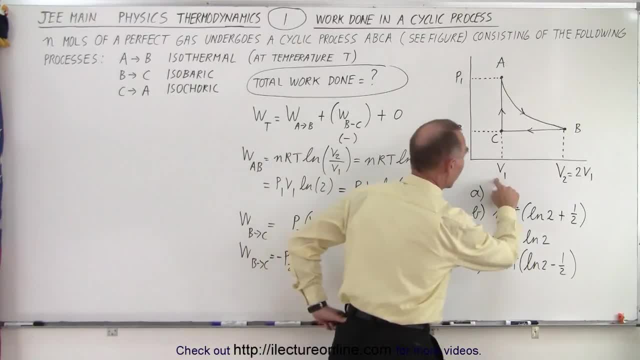 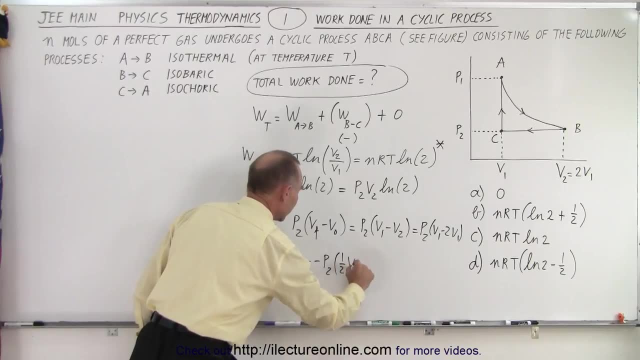 a half V 2, right, because when we go here, V 1 is half of V 2, so this can be written as minus P 2 times a half V 2. and why did I do that? because P 2- V 2 is the same as n RT, right? n RT is P 1- V 1 or P 2- V 2, so this can be. 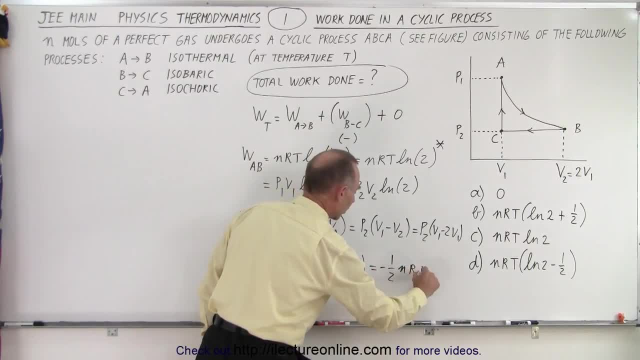 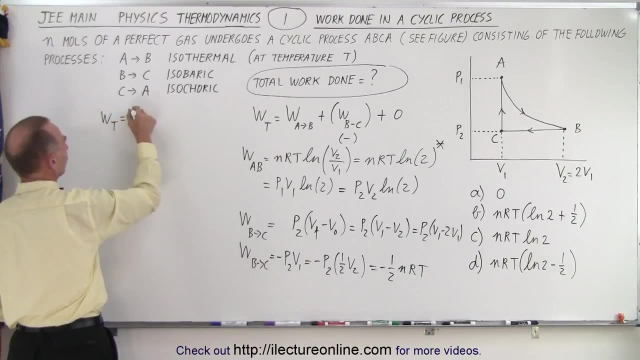 written as half V 2, because when you go here V 1 is half of V 2, so this can be written as minus one half times n r t. so now all have to do with attitude together. so now we have work. total equals the work from a to b plus the work done from b to c. so going from a to b i have 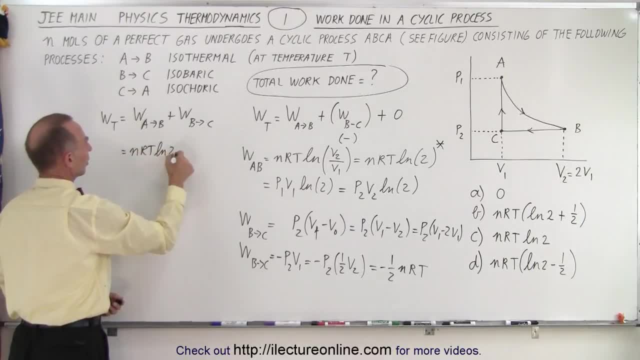 this is equal to n r t times the natural log of 2, and the work done from b to c is minus one half n r t. so when i factor out an nrt, the work total is equal to n r t times the natural log of 2, minus. 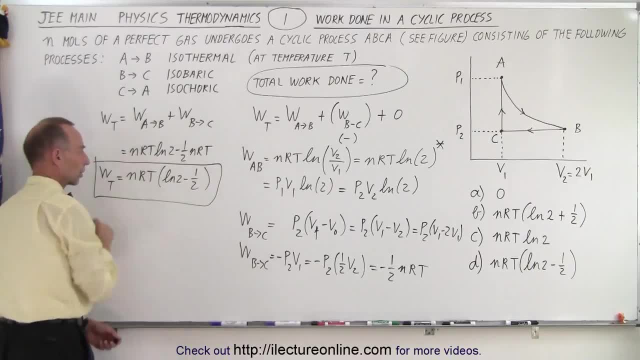 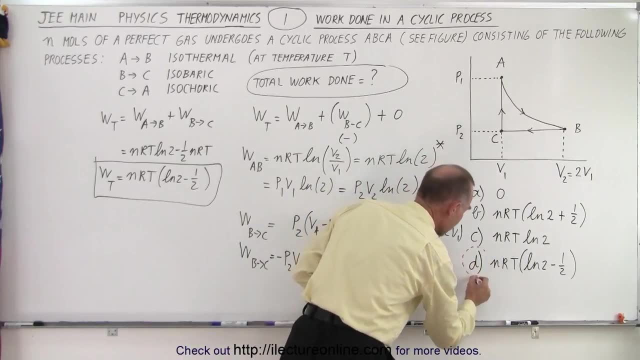 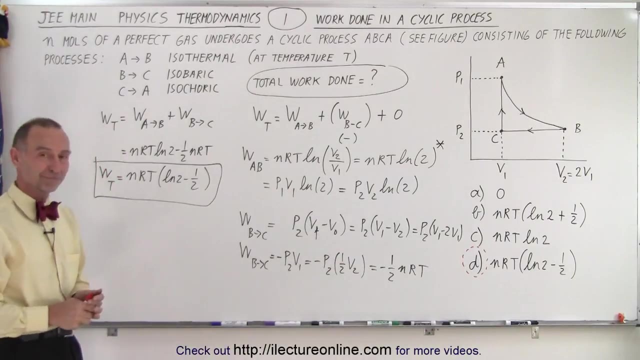 one half and that is how we find the total work done. now, when we take a look at the answers, notice it is answer number d. that's the correct answer. nrt times the natural log of 2 minus a half, and that is how it's done. 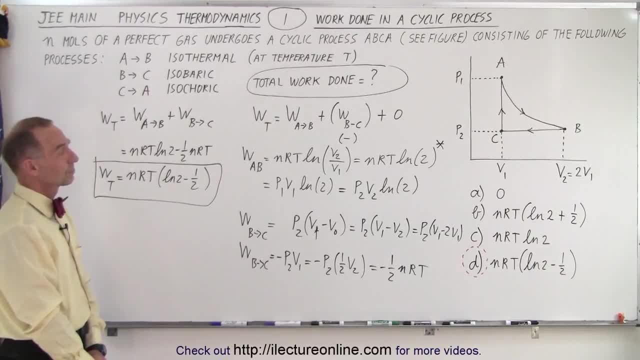 did i do that in three minutes? probably not. huh, five and a half minutes. of course, i did a lot of talking. well, it's a good excuse. i'm explaining things, so it takes a little longer. this could be done in about three minutes if you really work hard, if you understand the concept. 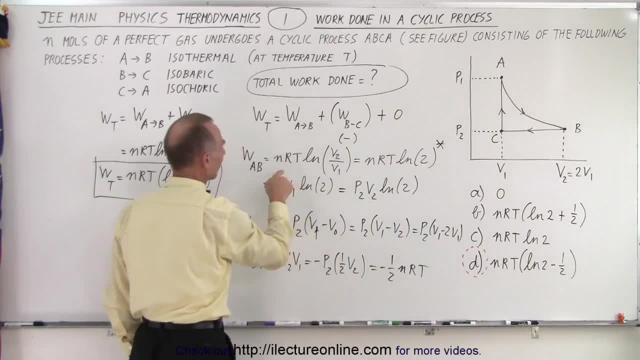 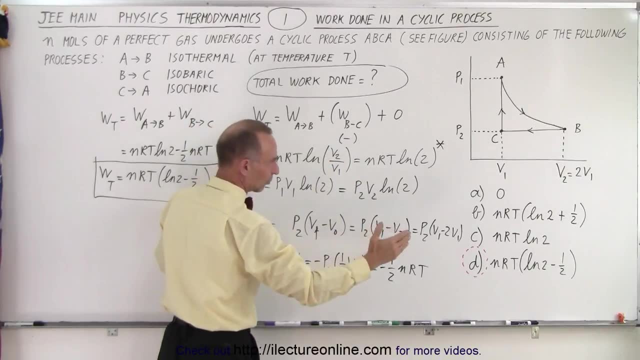 of finding the work done. you realize that this can be explained by these three equations: nrt times the natural log of the ratio of the volumes, which in this case is a two to one ratio, because it expands to twice the volume. you can also reuse p1- v1 instead of nrt, or p2- v2. 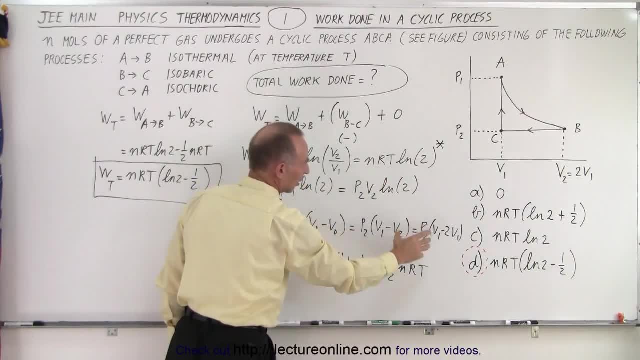 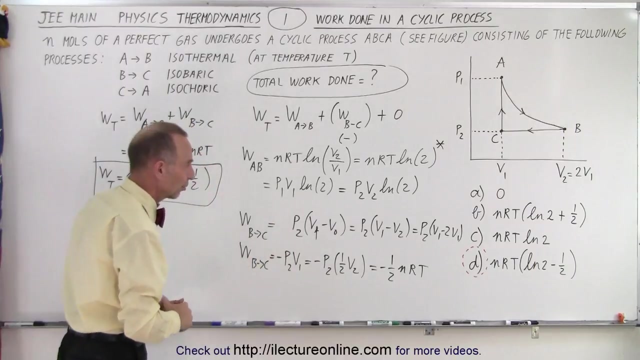 but essentially, since the answers are expressed in nrt times, the natural log of 2- we definitely want to. you can see that disappears in these three answers. you know it's not going to be zero because it can only be zero if there's no area inside the cycle. since there's an area there, it cannot be zero. 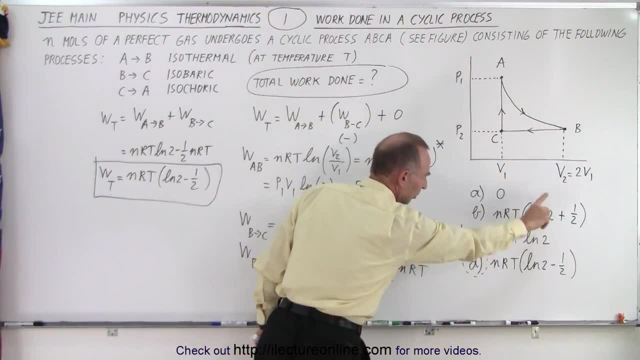 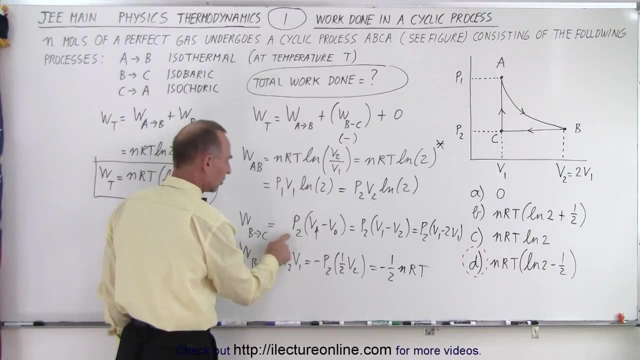 so we see that we want to use nrt times, the natural log of two. but how do we get the rest of it? well, in that case, work done from b to c can be found to be the pressure times. the change in the volume, v final minus v initial- v1 is smaller than v2, so it's a negative quantity, and so we end up with.